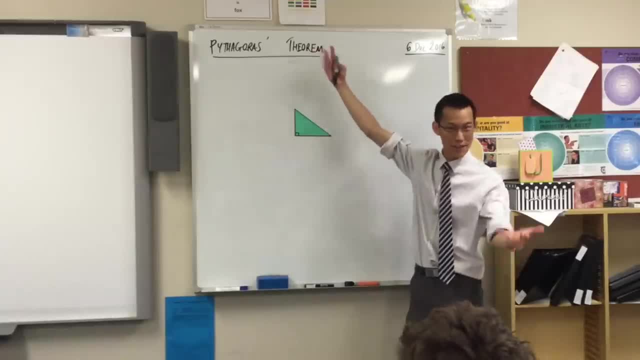 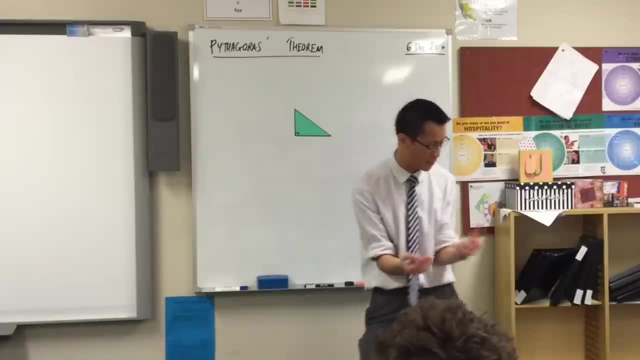 So here's what I'm going to do. This theorem, this property, this result relates these three sides together, So I'm just going to give them some names. Do you remember in algebra we gave numbers names when we didn't know what they were. 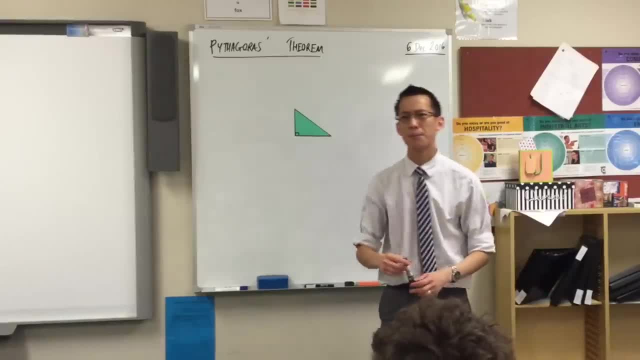 What was the point of doing that? Why is that useful? Yeah, Truan, Just in case you wanted to write the name of the angle. Yeah, like an angle or a side or any kind of unknown value. I'm going to give these guys names A, B and C. 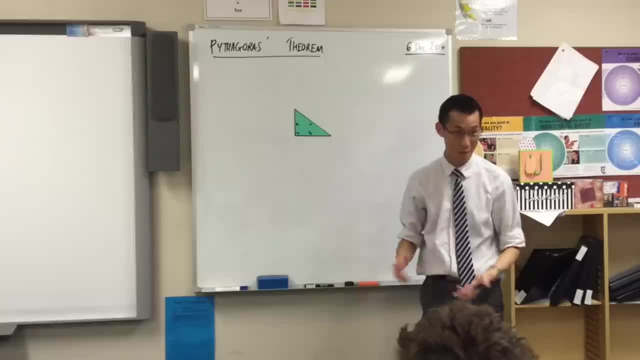 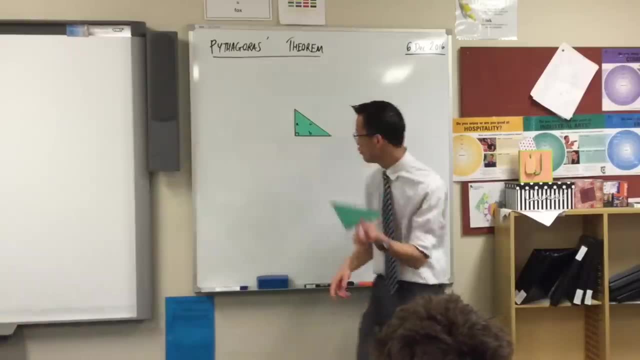 Not very original, I know, but at least that way it won't be hard to remember them. Now, A, B and C: they're the three sides of this triangle, And what I'm going to do is I'm going to put a few more copies of this same triangle up on the board. 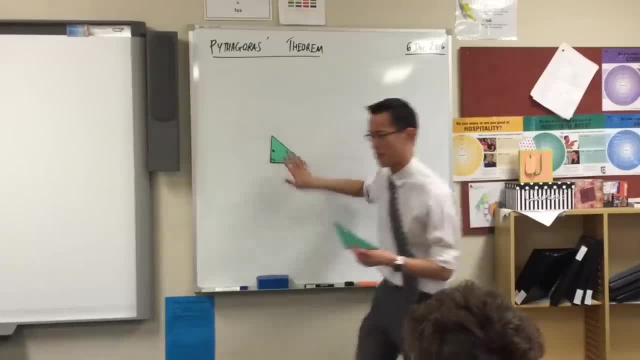 so that I can make a bit of a construction, a bit of a shape. So all of these triangles are the same. I've got four of them, So I'm going to arrange them in a particular way that I want you to notice. 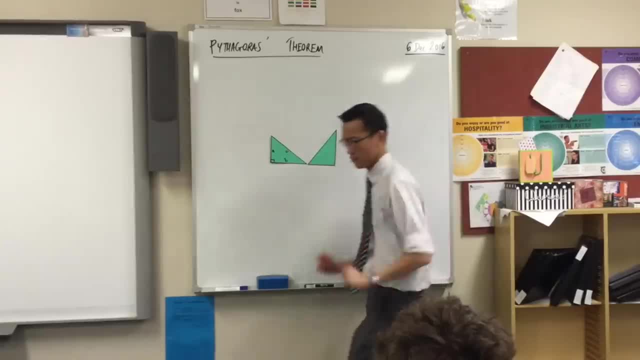 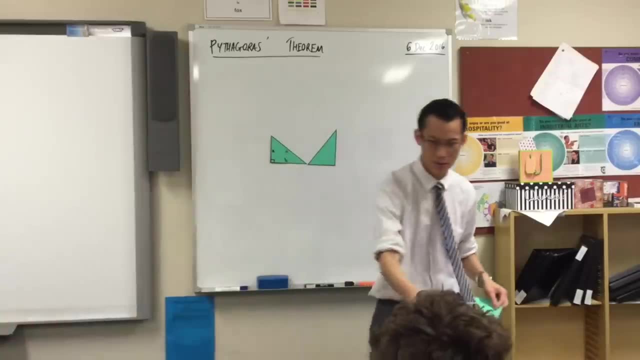 So I'm going to put this one over here. Good, I've got two more copies that are identical. Sorry, Tom, can you stick that securely on the back for me? I'm going to put this one, I'm going to spin it around a little bit like that. 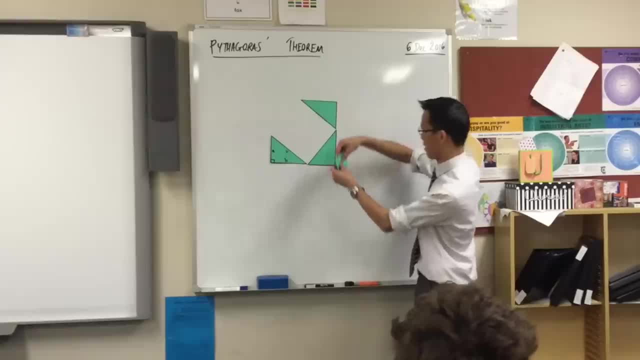 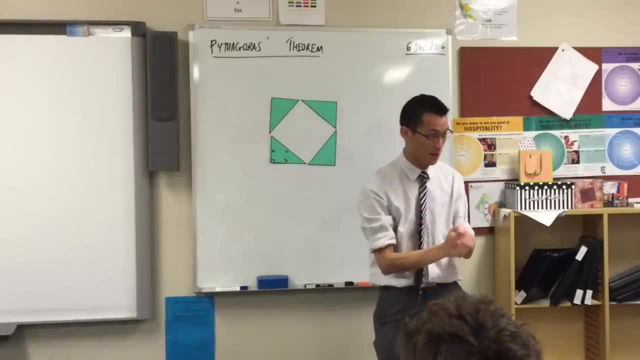 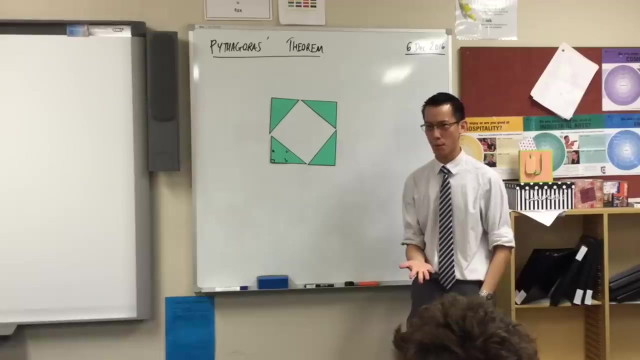 Okay, and the last one, Thank you, Okay, wonderful, Okay. Now I want you to look closely at the shape that I just made. By putting these four triangles together, I've actually made two new shapes. Can you see both of them there? 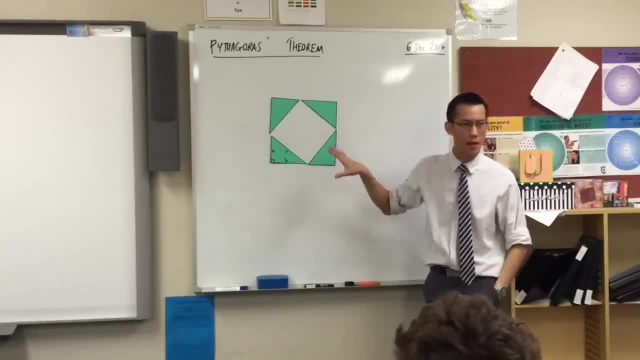 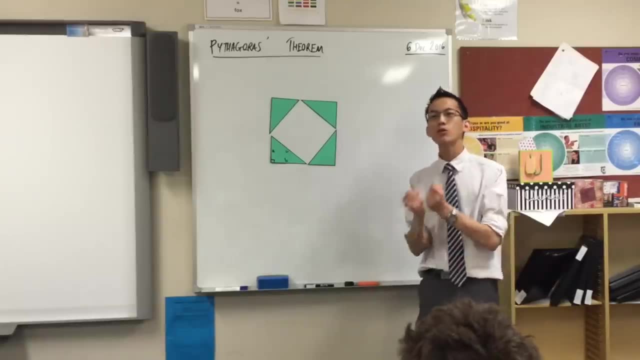 There's one that's big all the way around. What kind of shape is that Square? It's a square. Now just pause for a moment. Don't answer yet. just think about it. Apart from the fact that it looks like a square, how do you know that it's a square? 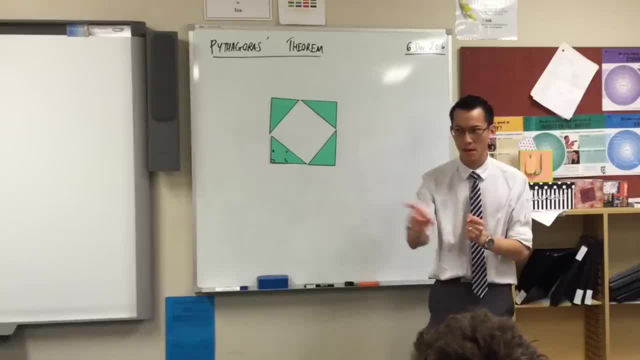 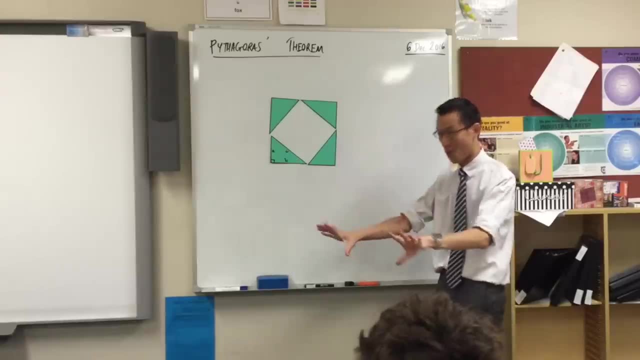 Think for a moment. think Hmm, Charlie, I saw your hand up there pretty quick. Why do you think this is a square? It's got four sides. Okay, number one, the first like requirement for a square. it's got to be a quadrilateral, so tick, all right. 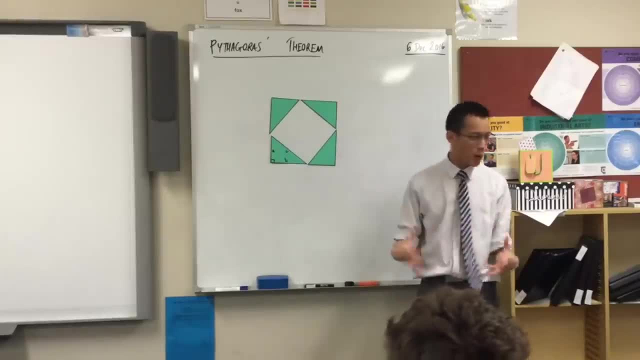 Nikhil, give me something else. Ah now, what makes a square a square? Wait, no wait- Is that the four sides are equal. The four sides have to be equal right Now, hold on a second. How did you know that the four- I mean, I know they look equal. 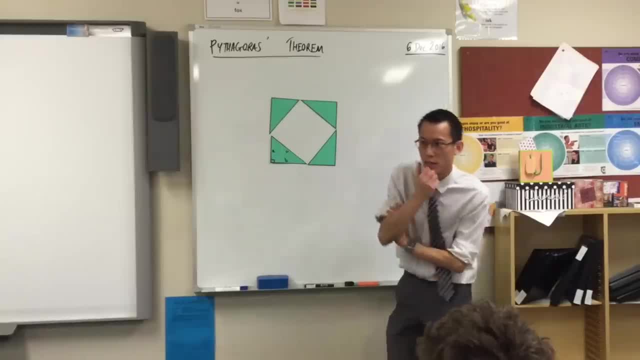 but how did you know that they were equal, Daniel? what do you think? The right angle on one of the shapes? yeah. This one here, Yeah, Okay, Now you remember. I said: all four of these triangles are the same, yeah. 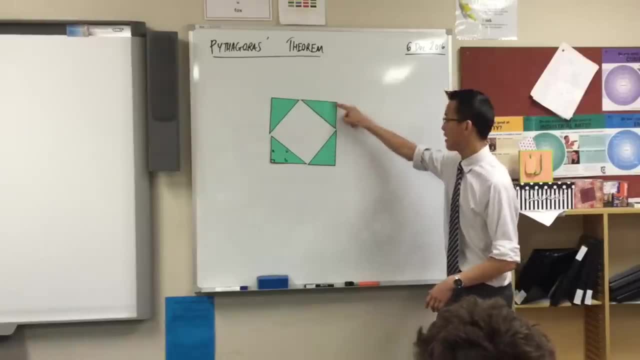 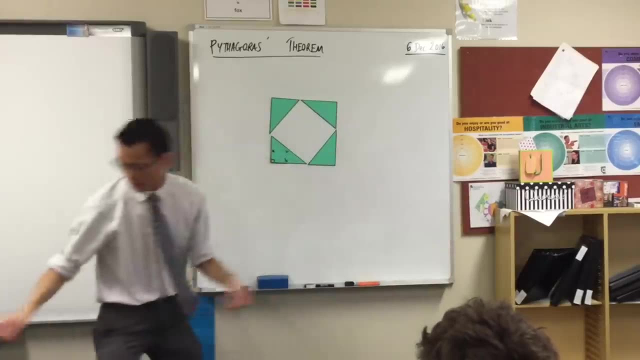 So I've got a right angle here, which means I've got one here and here and here. Those are important, but they still don't tell me that all of the sides right, like this one here. this is a side right. 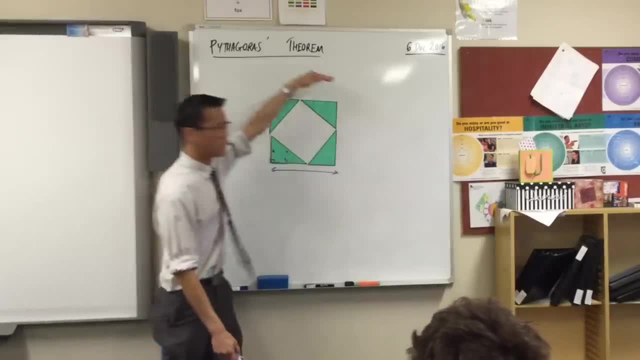 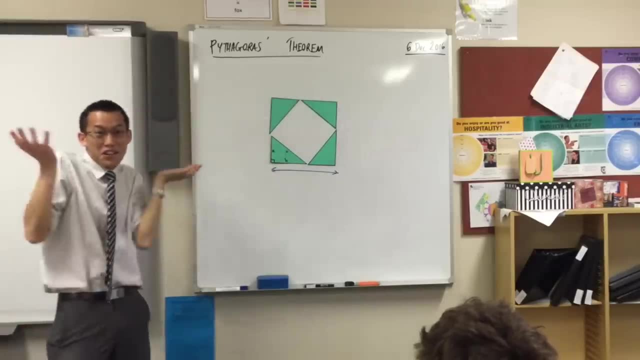 It doesn't tell me that that side is the same as this one, and this one and this one. Can anyone see how we can know? What do you reckon, Frank, Is this square? I'm trying to show that it's a square, though. 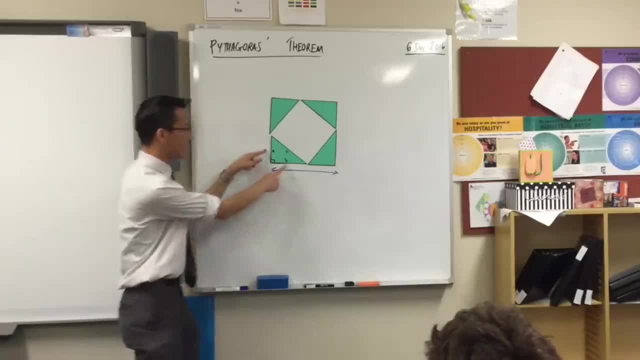 I know it looks a lot like a square. Let me help you out a little bit. okay, What did I name these sides again, A and B? yeah, So if this is B here, this one's slightly longer than A. Can you see it right? 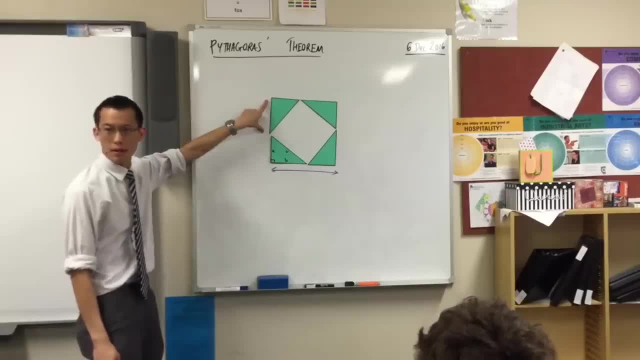 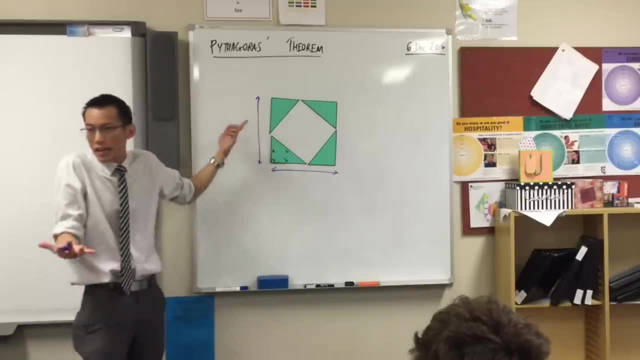 What's this side here, B, This is also B, right? So what's the height of my square? There's an A here and it's B, so you just add them together: A plus B, right? Are you happy with that? 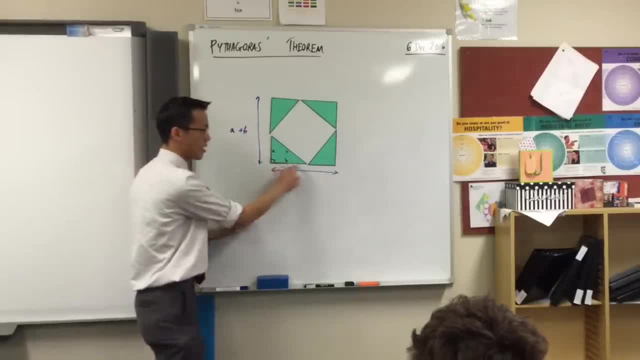 Now have a look at the bottom. Have a look at the bottom. Can you see I've got B here. What's this guy? A It's A. So what's this? A plus B, And you can do this all the way around the four sides of the quadrilateral. 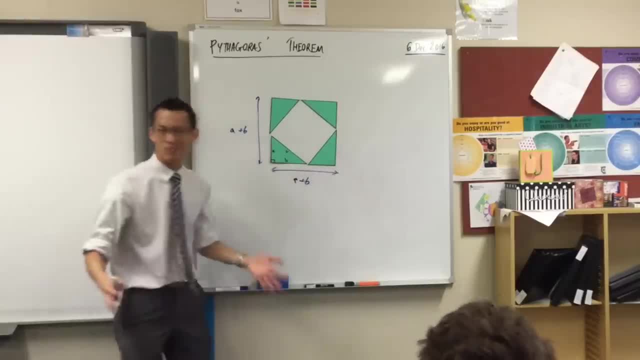 So you're like they're all the same, They've all got right angles, That's a square. okay, There's another square too. Do you see where the other square is? It's right there, stuck in the middle, right? 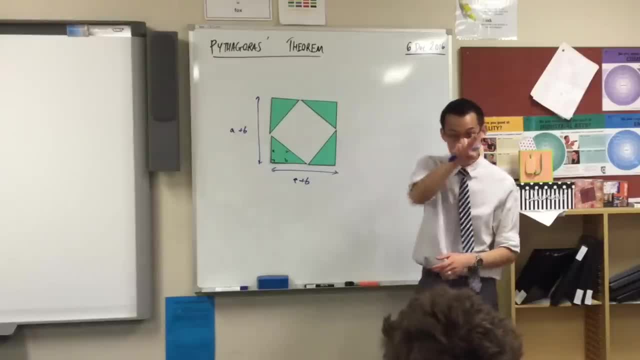 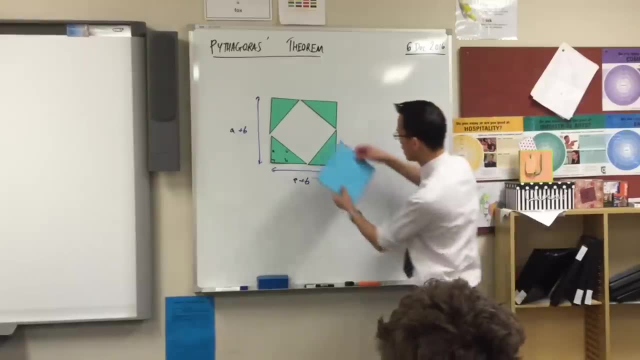 In fact it's so important. I drew it as well, okay, So you can see here. I drew it as well, okay, So you can see. it's off at an angle bit of a funny angle, So it's in here. 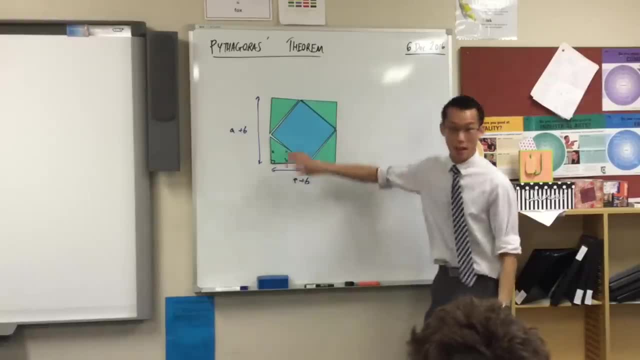 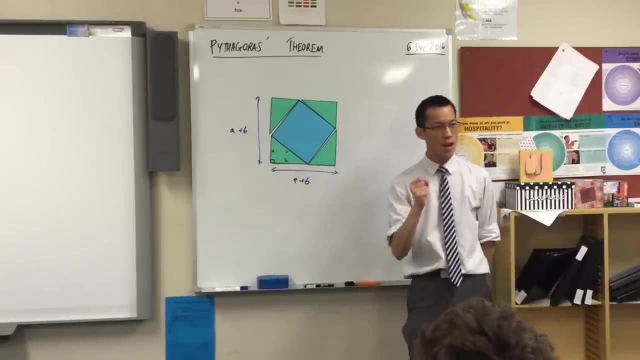 Okay Now, Pythagoras' theorem has a lot to do with this particular blue square. That's why I drew it for you. okay, I want you to think for a moment. What's the area We've done? area before: 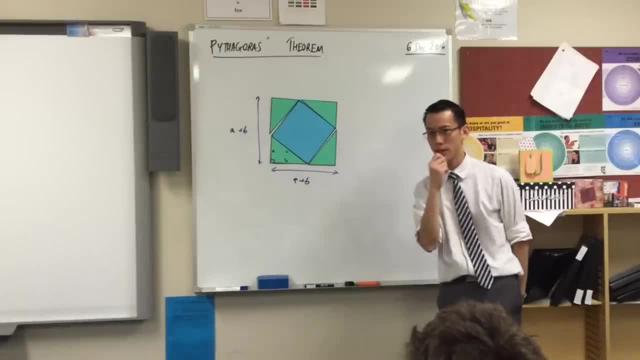 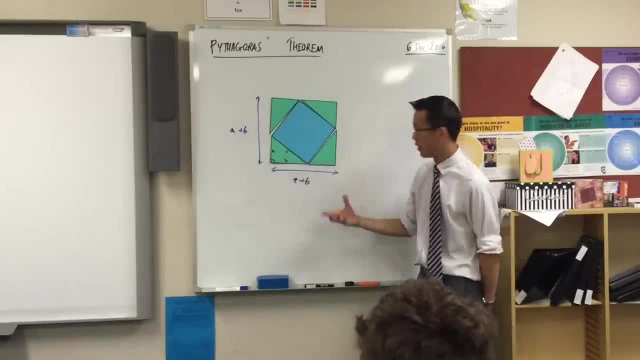 What's the area of this blue square? What do you reckon, Truman? C times C. Hmm, Remember? all of these four triangles around the edges are the same. This is C this side here. That means this is C as well. 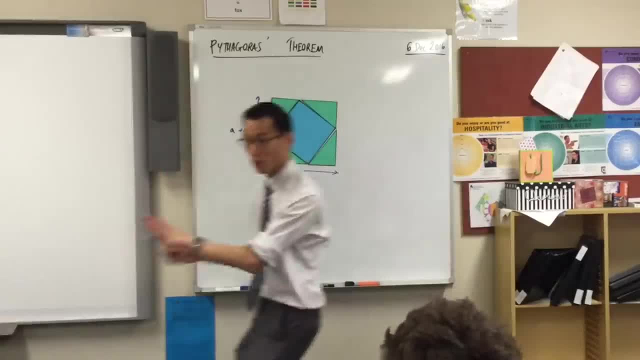 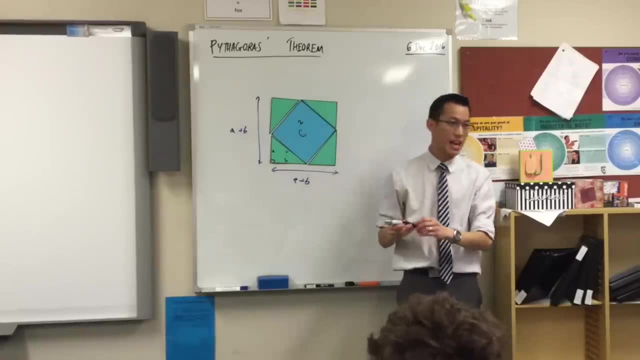 In fact, they're all C. okay, In fact, that's so important. I'm going to label this square. Let's do it like this C squared. Can you see that? That's the area. Now, I don't know what C is, but algebra doesn't care. 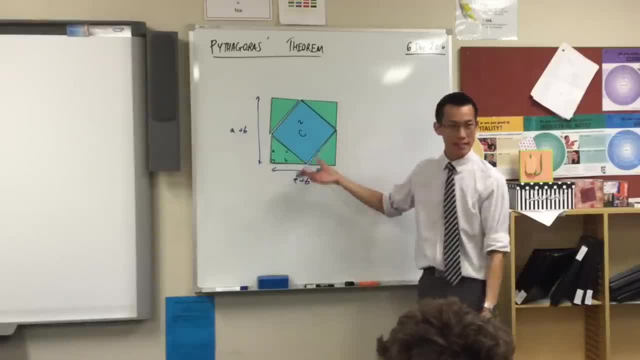 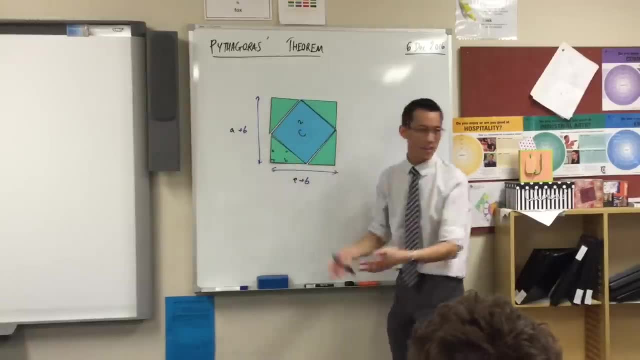 It's like: well, whatever it happens to be, it's that squared. It could be like 10,, which would make this 100.. It could be 7,, which would make this. what would that be? 49.. It could be 8,, which would make that. 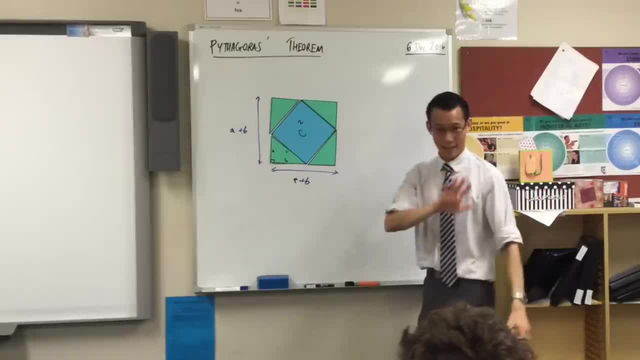 No, no, no, no, no. It could be anything. That's my point. Okay, Now let's just take this guy. I'm going to put C squared over here for a minute. Just hold on to him in your mind, okay. 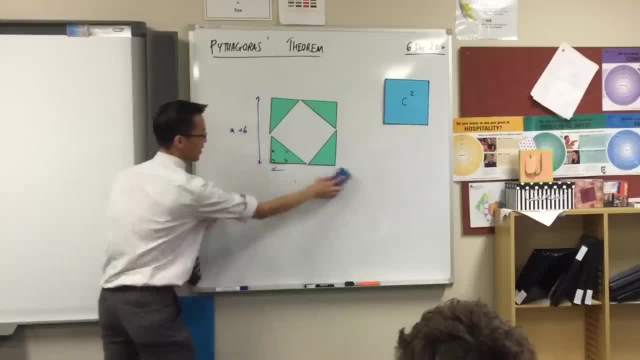 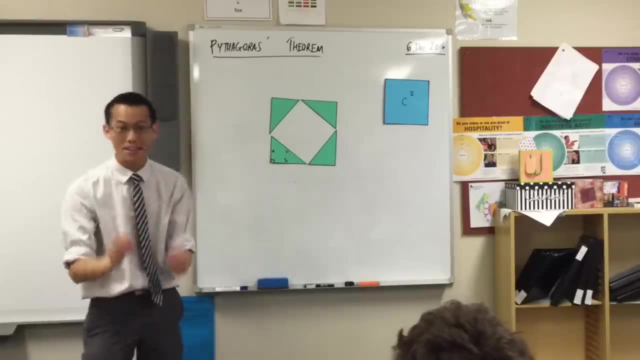 Right, I need a little more space. Now, what I'm going to do here. here comes the proof. That was just the setup. I'm going to just rearrange these same four triangles, okay, And I want you to watch the way that I do it. 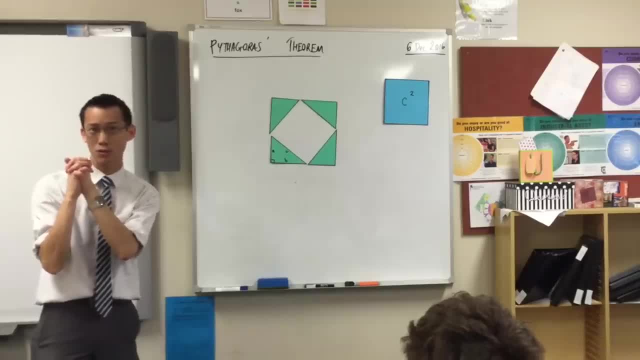 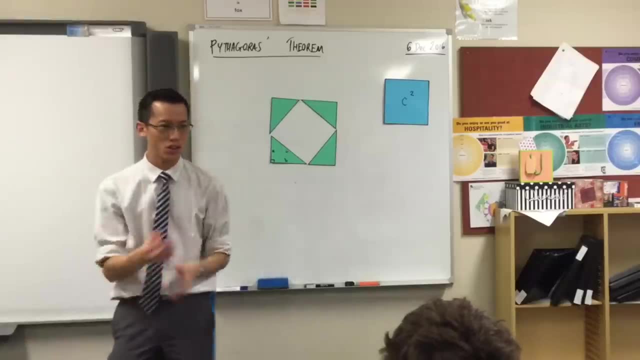 Um, Let's go back in term one or two. We learned about these things called transformations. We could change shapes, We could like, move them about in different ways, and they stayed the same. Do you remember what the three transformations were? 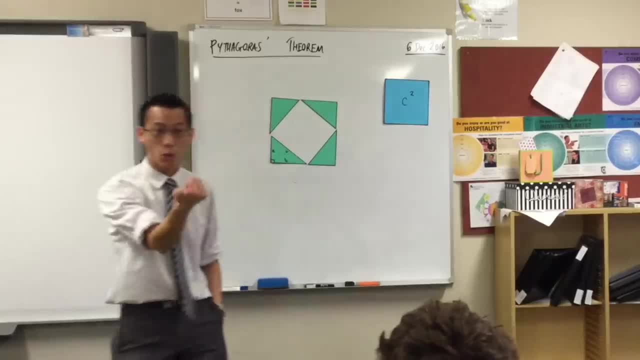 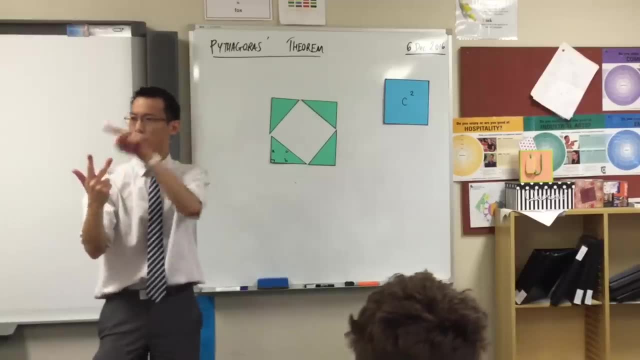 Any suggestions? Nikhil, can you give me one Slide, Slide or translate What's another one, Frank, Reflect, Reflect or flip. And the third one was Rotate: Rotate, okay, Or spin or turn right. I'm going to use two of those. 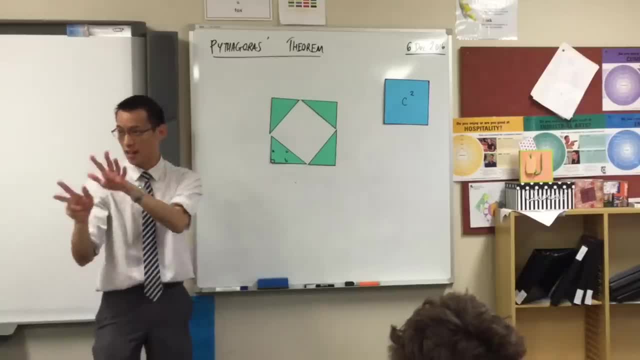 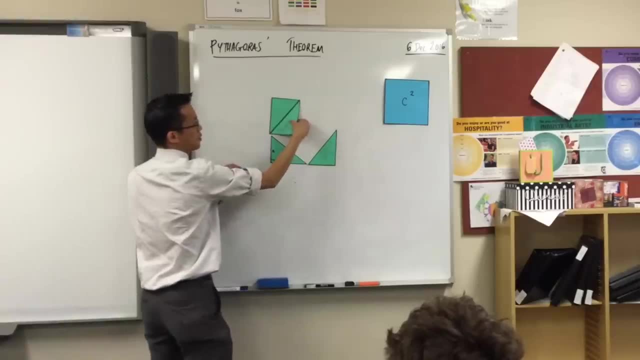 I'm going to use rotation and I'm going to use translation. That's sliding. Okay, watch, I'm going to take this guy. I'm going to rotate him around like this Spin, So he's over here. Okay, Are you happy with that? 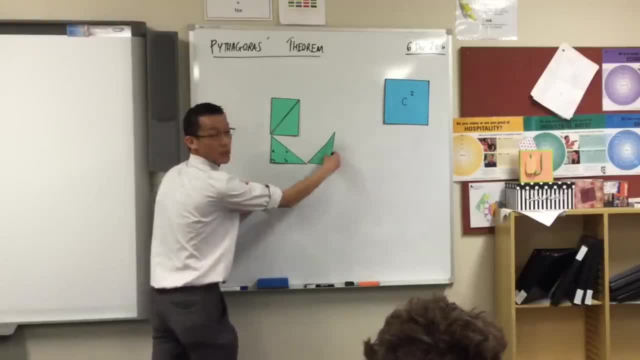 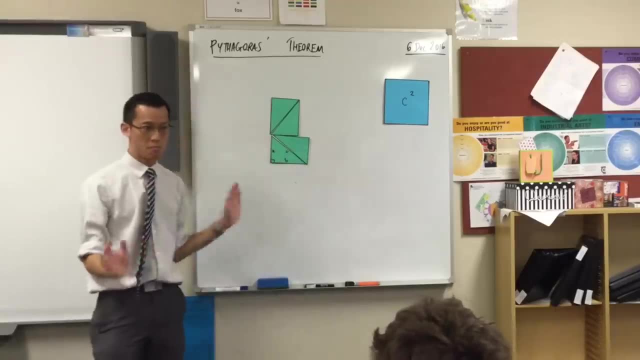 You see how I did it. Okay, I'm going to do another rotation, This one I'm going to rotate in a similar way, Anticlockwise, Around, like that. No shapes have changed, They've just moved positions a little bit. 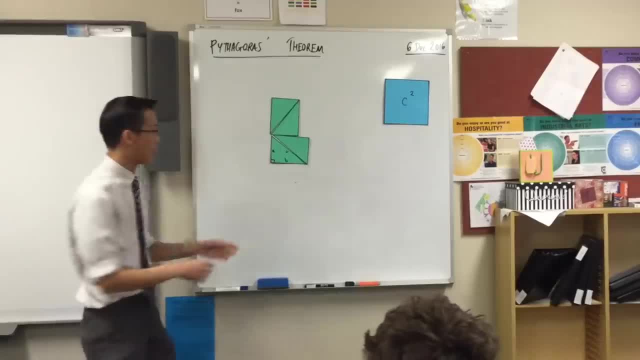 Okay, Now I'm going to do my translation. I'm going to slide, I'm going to take this shape. What's this shape now that I've made? It's a rectangle. It's a rectangle. I'm going to take the whole rectangle. 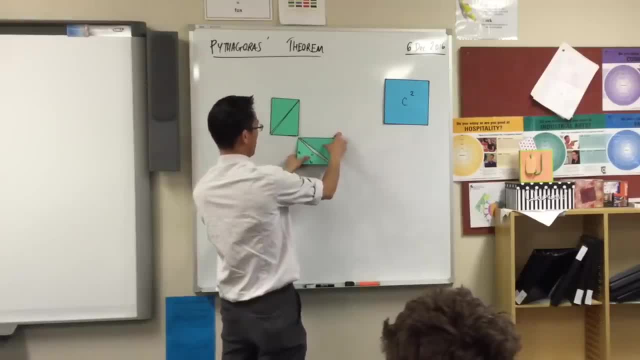 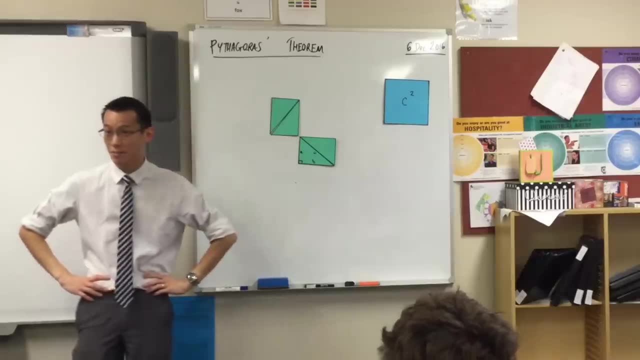 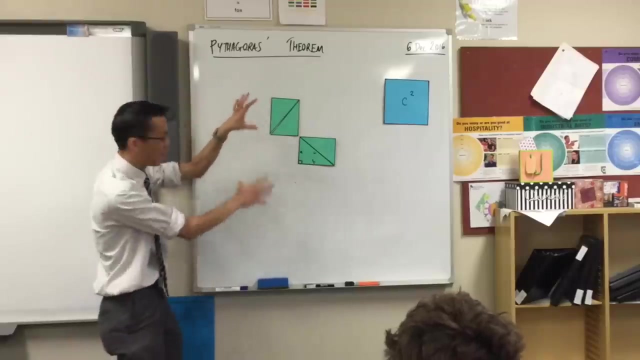 And I'm going to move it over just a little bit. Okay, Now this is my new setup. Still the same four triangles, But again I've made some other shapes that you can kind of see around there, right For starters. can you see, I've made this guy over here. 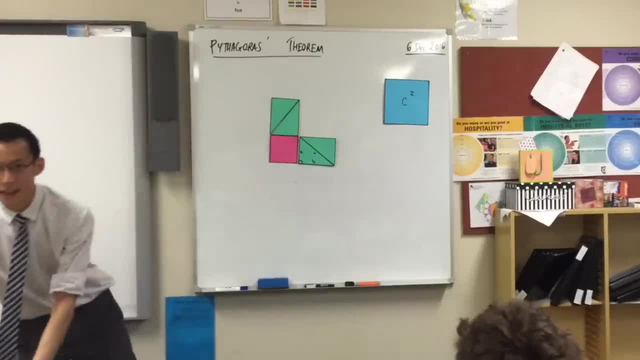 You see this guy. What kind of shape is that Square? It's a square again, But it doesn't just look like a square. Okay, How do you know it's a square, Christian? what do you reckon? Because both sides are A. 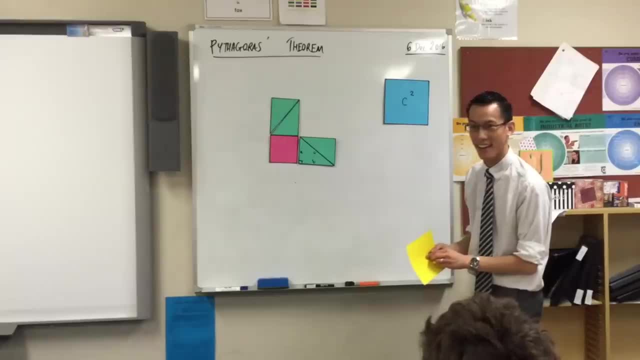 Yeah, very good, See, I think we've got this one labeled A And because these triangles are all the same, this is also A. Okay, And there were also all those right angles I talked about before, But that's the other square, the only square. 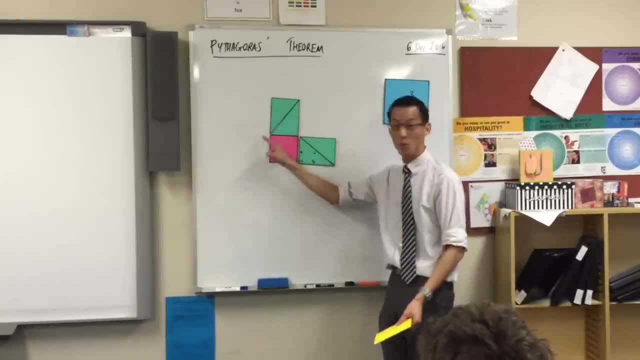 There's this one here. right, You see that, Are you with me? Okay, Now, what are the areas? Which one? What are the areas of these two triangles? I don't know, I don't know, I don't know. 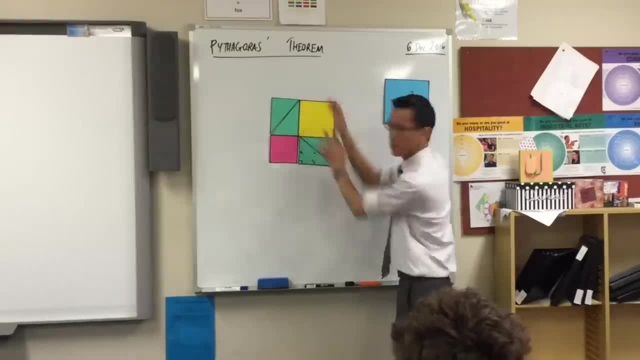 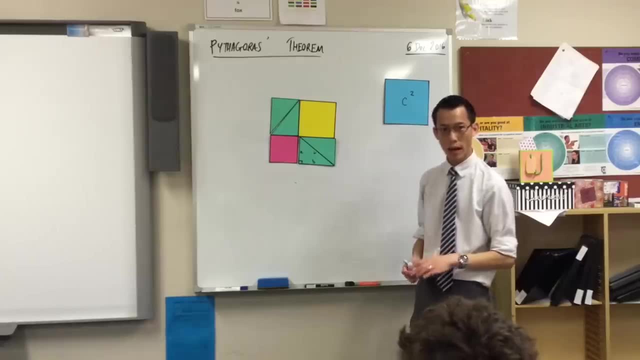 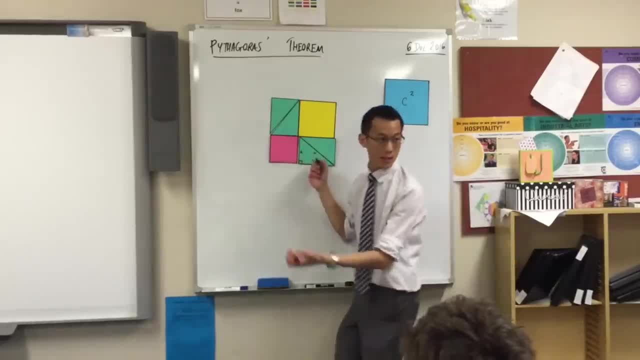 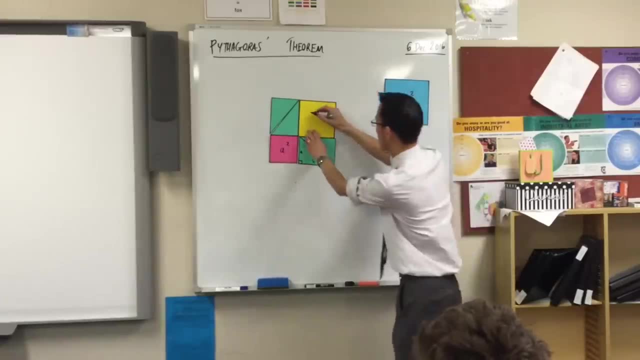 Well, let's do the first one first. It's A Times, A Times A, Which makes it A square, A square, Right. How about this one over here? B times B, Yeah, B times B. So it's. 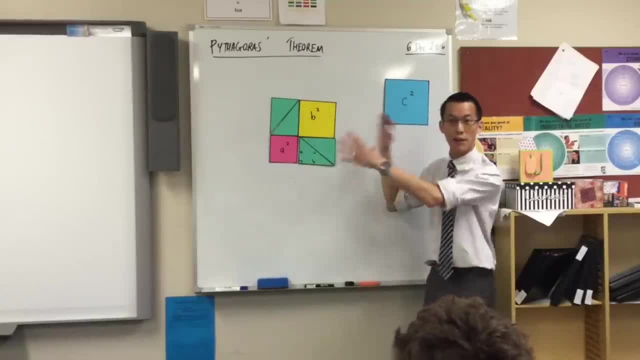 B squared, B squared. Okay, So I've got these two cool extra squares, But then have a look, Now that I've put everything together. what is this big shape that I've made A square? It's another square. In fact, it's not just any square. 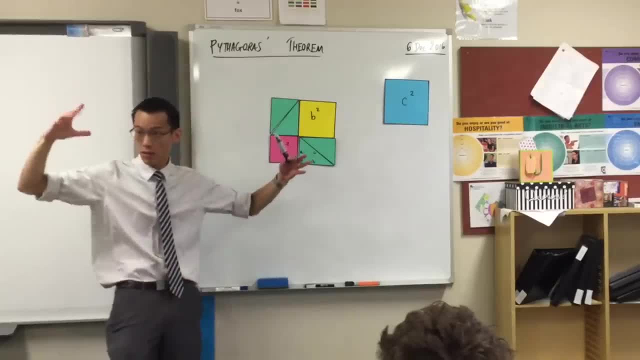 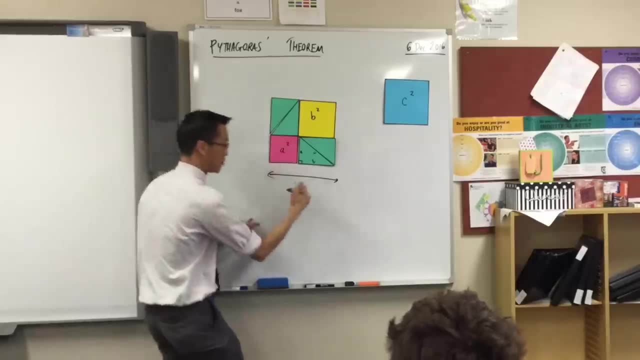 Isn't it the square I saw? Yeah, The one I started with, The big one. Have a look. What's this width across the bottom? It's A plus B, right, And you can say the same thing of the height, can't you? 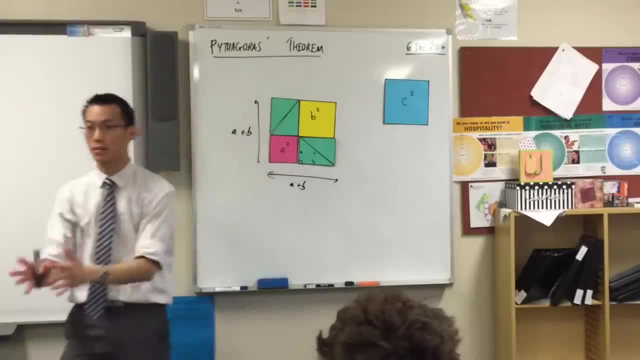 So, in other words, the two squares I made, the two big ones, were exactly the same square. Are you okay with that? Okay, Now, let me just draw that square over here. It looked like this: if you recall Something like this: 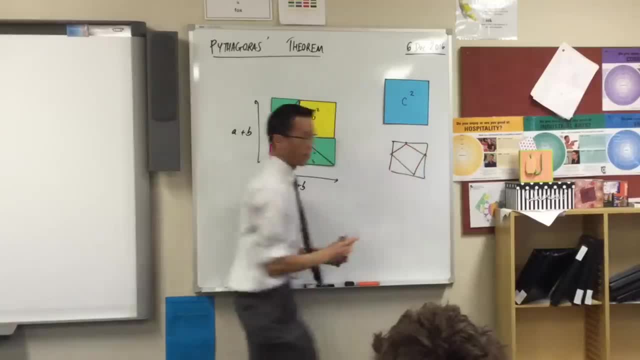 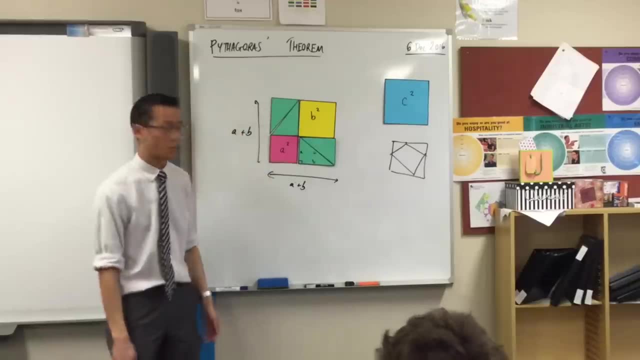 Here we go. Do you remember that? Yeah, Yeah, Yeah, Yeah, Yeah, Yeah, Yeah. Okay, Here comes the finish. These four triangles, they started off really important, okay, But I'm going to take them away from both of the squares. 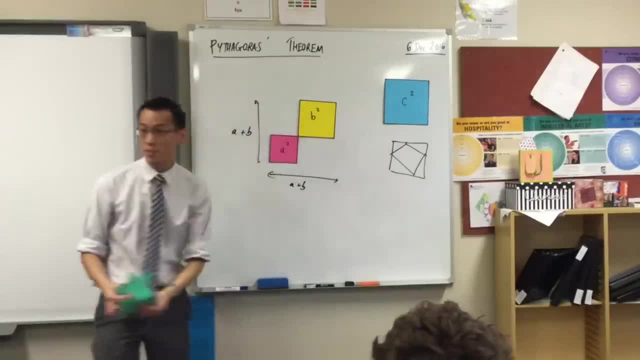 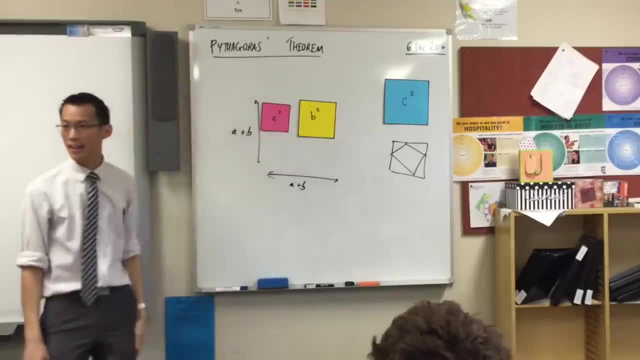 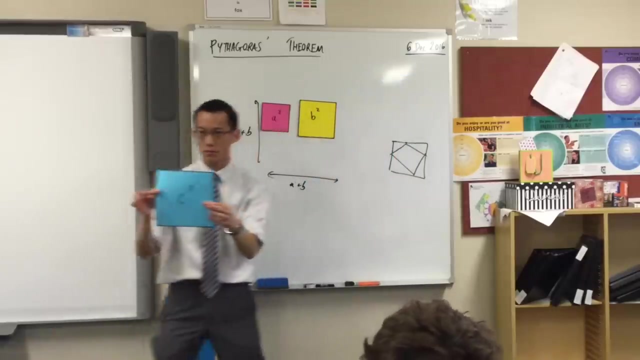 There we go. That just leaves me with those bits right Now. these are the leftover parts, right? Take away the four triangles, okay, But look, I've got these two. They were the leftover bits In the first place. the leftover bit was this whole square. 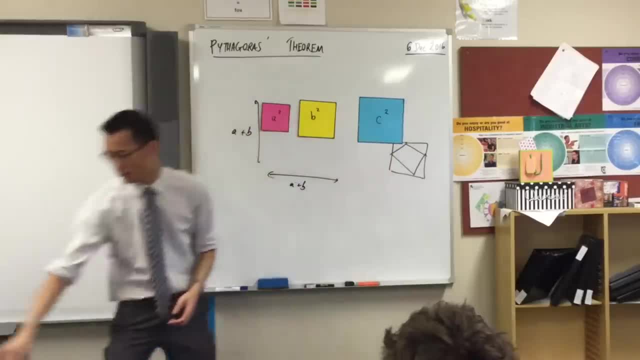 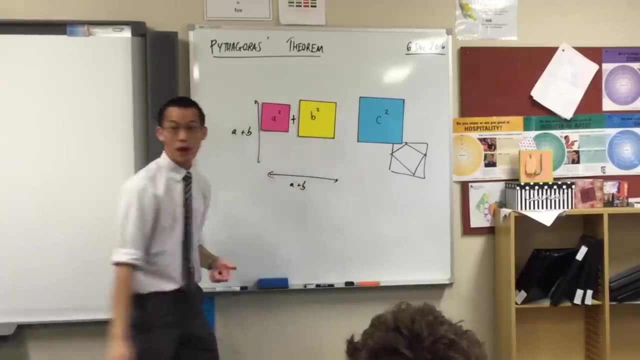 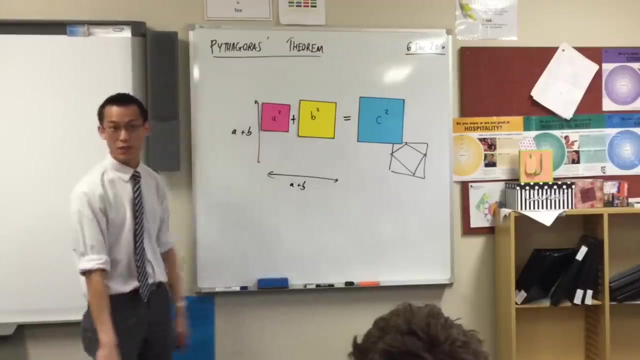 Do you agree? So, therefore, what Pythagoras' theorem tells us is that all of these sides, they're related. in this way, If you add these two gaps together, the leftover bits of the square, they're the same as those leftover bits of the square. 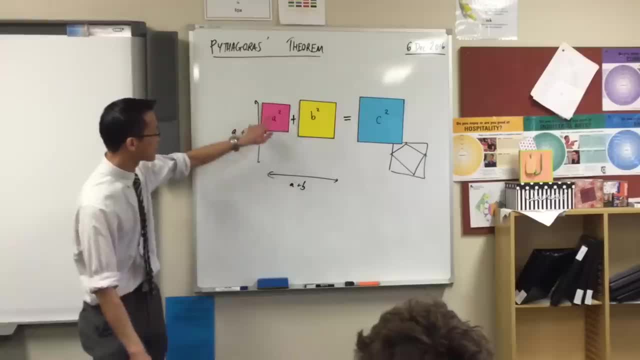 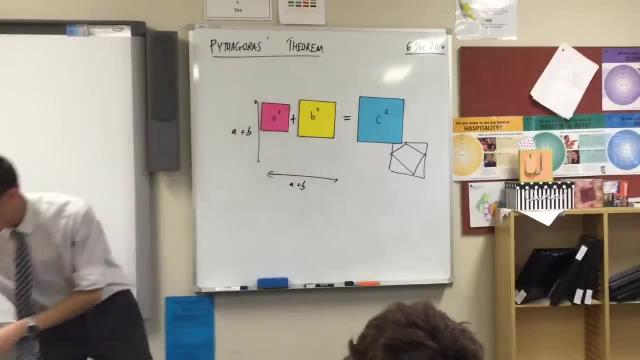 I've just rearranged them a little bit, okay. And this one, two, three. this is what we call Pythagoras' theorem, If you've got any right-angled triangle, okay. Now I want you to open your book up again. 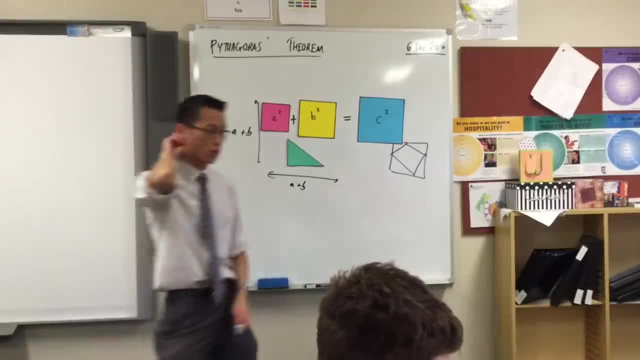 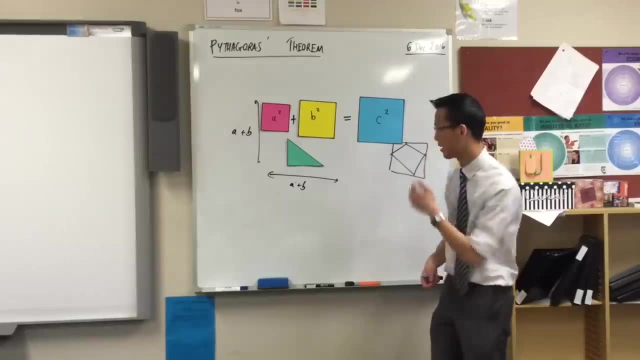 Okay, If you didn't draw your triangle with a ruler, I'd like you to draw one with a ruler. Maybe you need to borrow from a pen, okay, And what I want you to do is I want you to measure those sides. 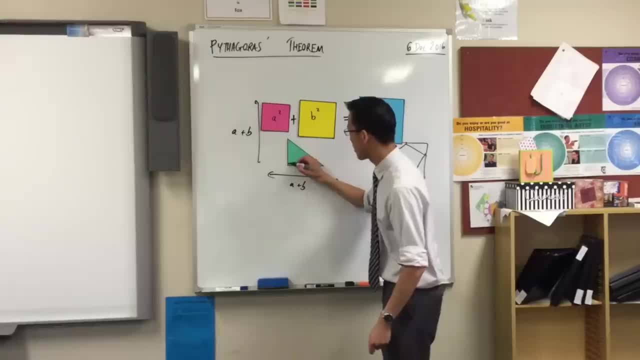 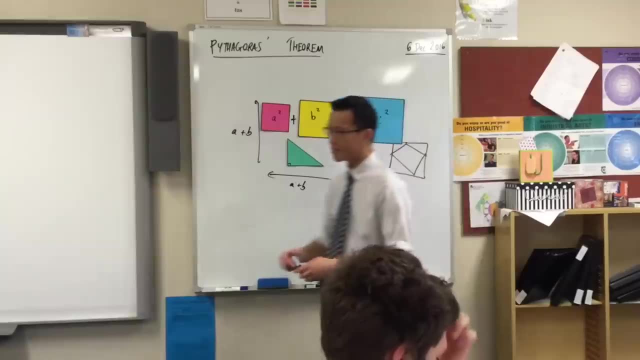 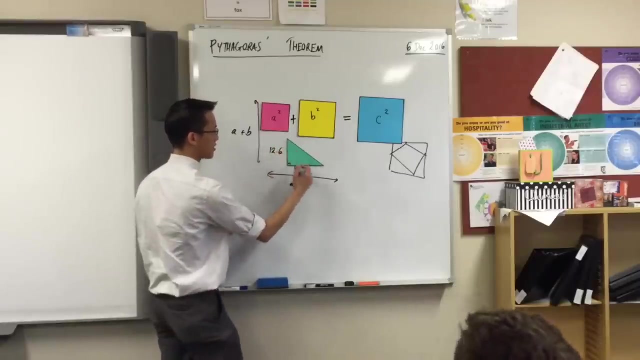 That's really important that the sides meet at a right angle, like that. If you measure them, for example, on mine, what I did was I measured out all of these sides. Okay, I think what I? I think this is 12.6 centimetres and 16.8 centimetres. 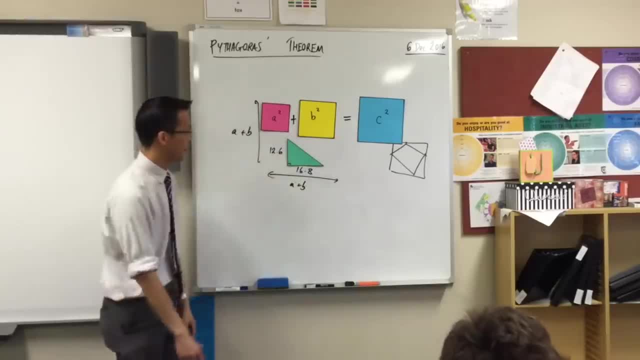 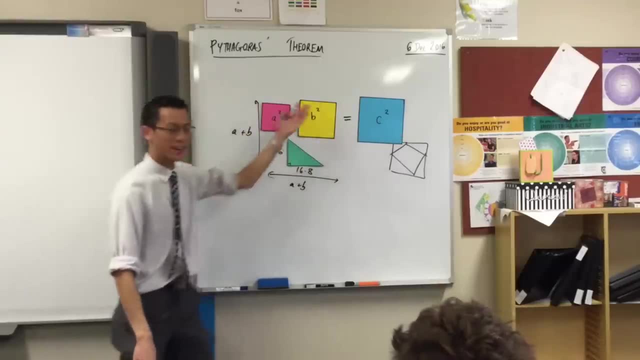 You can work out what the last side is, the longest side. You can work it out by just measuring it, by putting a ruler on it. But you can also work it out using this relationship here, That a squared plus b squared will equal this last side here squared. 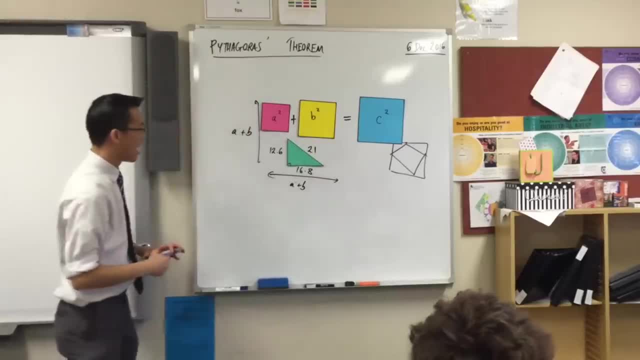 In this case it's 21.. Okay, A really famous one. If you haven't, If you have drawn like a triangle and it's a bit messy, you can draw a triangle like this. It's not going to be messy. 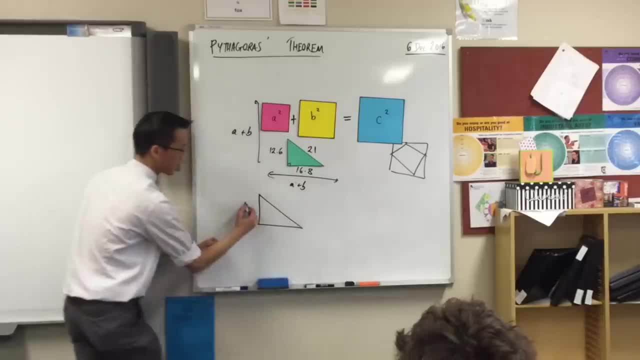 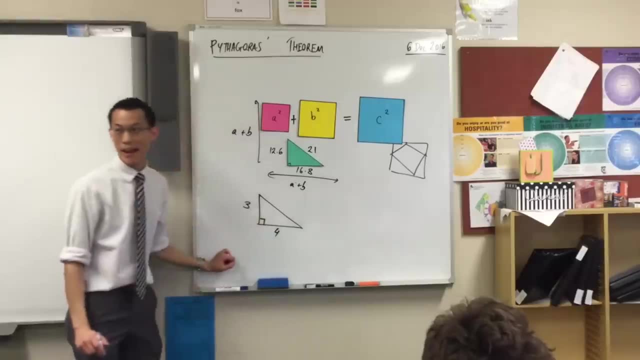 You can draw a new one. Make it like this: This is a very famous one. If you've got one, that's One edge that's three centimetres and one edge that's four centimetres, so long as they meet at a right angle, this last one should be five. 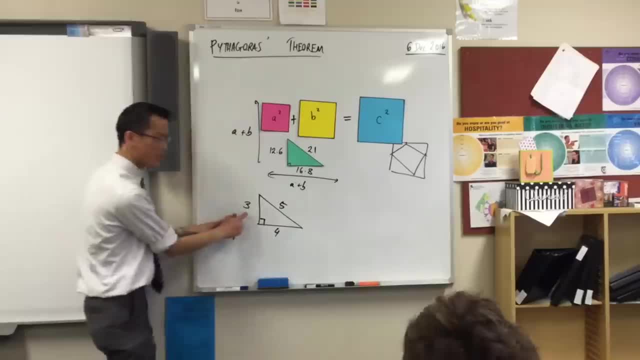 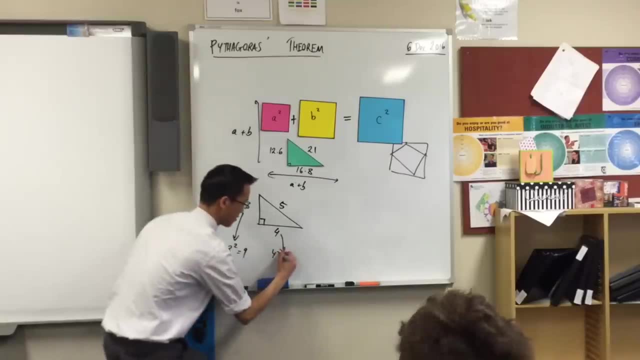 You can't help but make it five. Here's why Watch: What's three squared Nine: Three squared is nine. What's four squared Sixteen, It's sixteen. And if you add these two together, you get 25.. 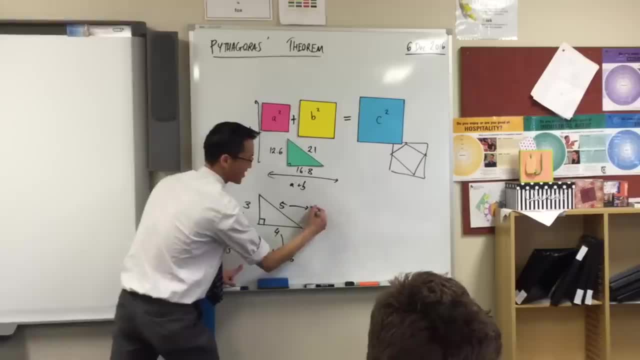 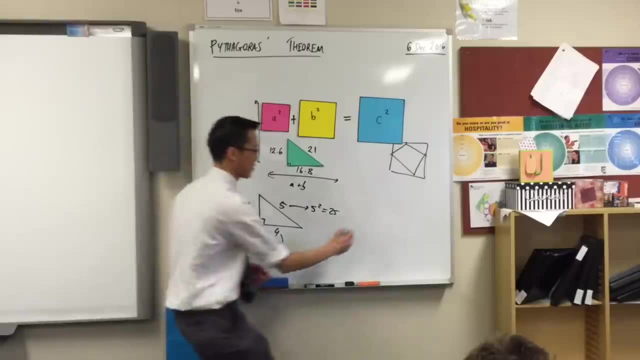 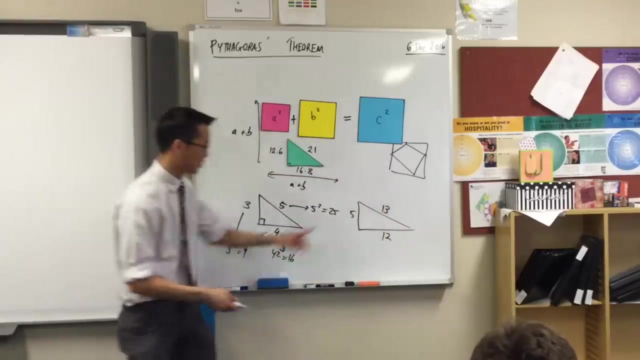 25.. Which is Five, Five squared Right. Very good, So you can do this with any set of triangles. Another famous one is five centimetres and 12 centimetres and 13.. You can do the squares yourself and you can find out: 25 plus 144 is equal to 169..